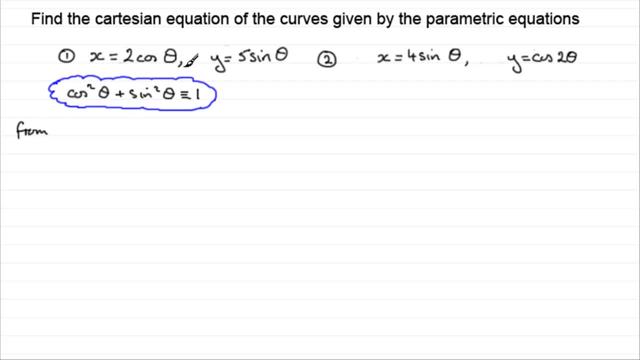 sides by two. we can see that from. well, we better number this, I think lets say number 1, and we will call this number 2.. So from equation 1, we can see that cos theta equals x over 2.. And from equation 2: here, if we divide both sides by 2, we can see that sin squared theta is equal to x over 2.. And from equation 2: here round this would be final. We have to divide both sides by 2 over expansion. 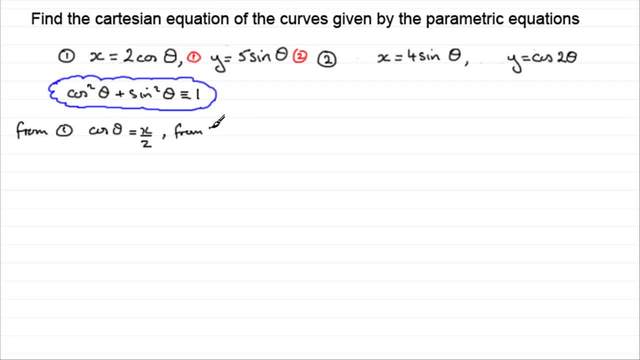 by 5, we can see that from 2, sine theta equals y over 5.. And okay, I might have been thinking this, but if I was writing it down for real, I would say something like: since cos squared theta plus sine squared theta equals 1, notice how I've changed the identical sine to an. 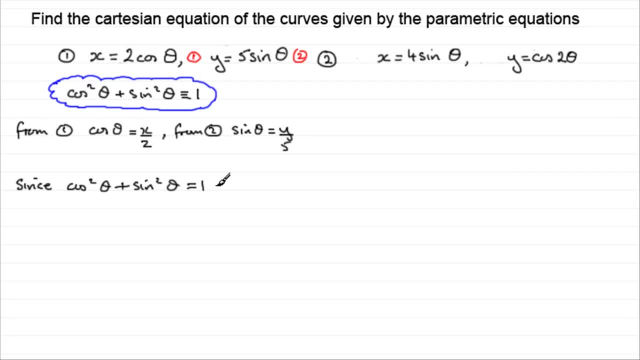 equals here, because we're getting a Cartesian equation. Then if I square this, we're going to have x squared over 4, and I can substitute it in here. We would therefore have x squared over 4, plus and for sine squared theta. if we square this, we've got y squared over 5. 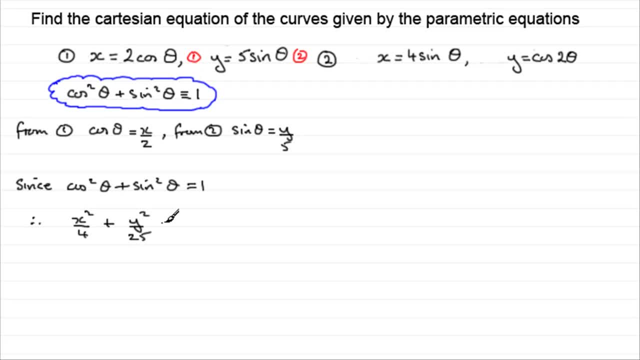 squared, which is 25.. And that would equal 1.. And I could leave it like that if I wanted to. I could times both sides by a number that 4 and 25 go into, That's 100.. If I times this, 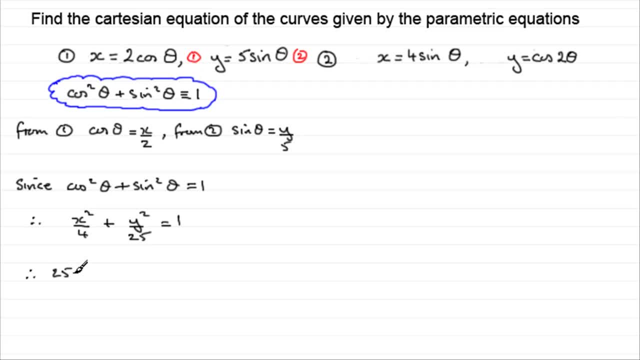 by 100,. I therefore end up with 25x squared, times this by 100, and I get 4y squared, And then the 1 by 100 just gives me 100.. Either way, any of these versions, I'm sure, would. 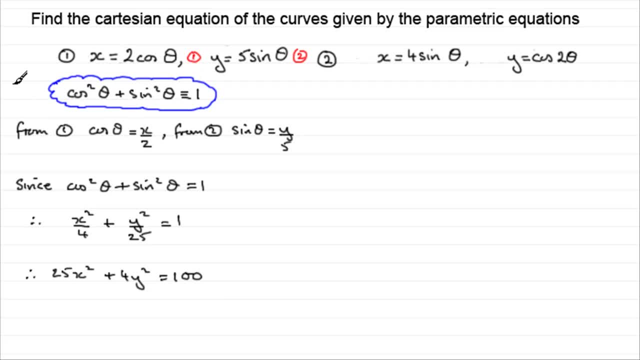 do. Okay. well, that gives you hopefully some idea on handling equations, Question 1.. You might like to have a go at this one. Try and think of some identity that links sine theta with cos 2 theta. Okay, well, let's see. How did you get on, Did you? 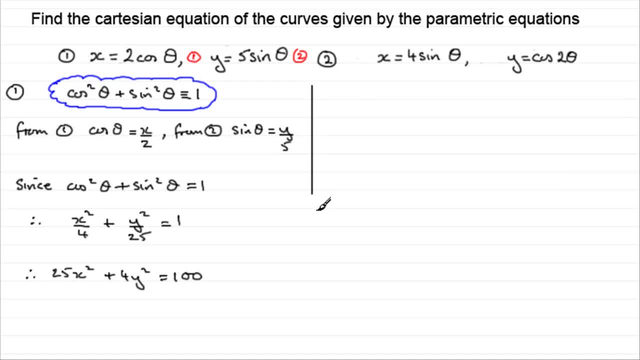 come up with that identity. Let's just come down here. So for number 2, what did you think of? Well, we've got to turn our attention to cos 2 theta. Why is cos 2 theta? Well, Do you remember that cos 2 theta was identical to 1 minus 2 sine squared theta? 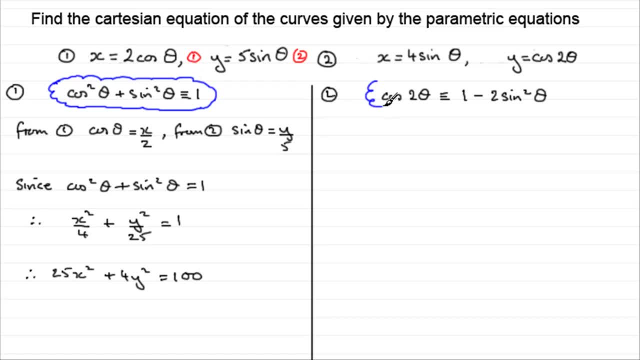 Okay, a well-known identity. So that's what I would have basically been thinking about. So, knowing that I'm going to head towards that, I want to label my equations. Let's call this 1 and this one number 2.. And I would say that from 1, we need to make sine theta the subject. 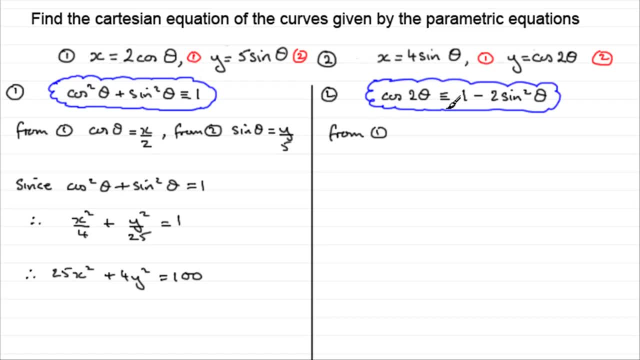 So from 1, if we divide both sides by 4, sine theta equals x over 4.. I don't really need to do anything with this, I've got it here. I'd remind the reader what equation I'm using. So I'd say: since cos 2, theta is equal to. 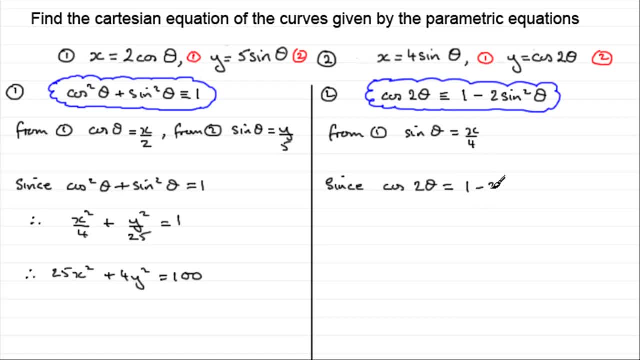 change the identity. So it equals here 1 minus 2 sine squared theta. I would therefore have: and in place of cos 2 theta I'd write the y, And it would equal 1 minus 2 times sine squared theta. 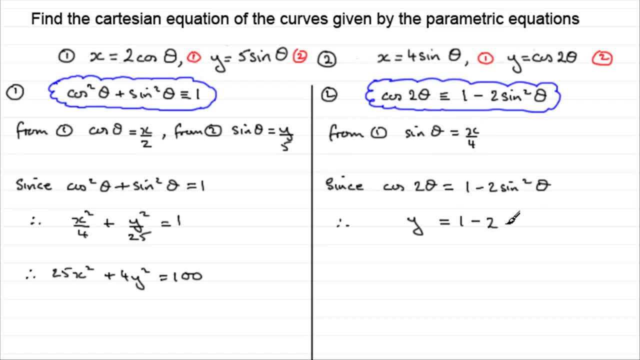 So I'd need to square this term and I'd get x squared over 4 squared, which is going to be 16.. The 2 sixteenths. now that cancels 2 goes into 2 once. That goes into that 8 times. 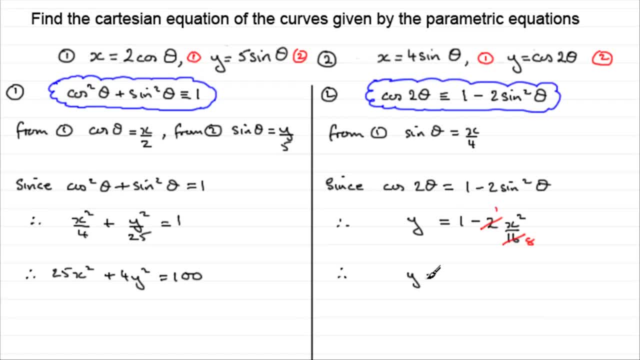 So I would therefore have y equals 1 minus x squared over 8. And I think I'd leave it like that. I've got it in the form y equals, so that seems okay, really. If you wanted to, you could times through by 8.. 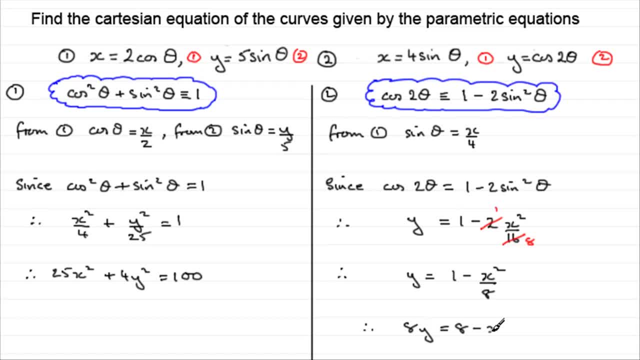 You'd get 8y equals 8 minus x squared. Give that as a version as well. Okay, leave it up to you anyway. Well, again, I hope that's given you some idea then of how you handle trigonometric types. 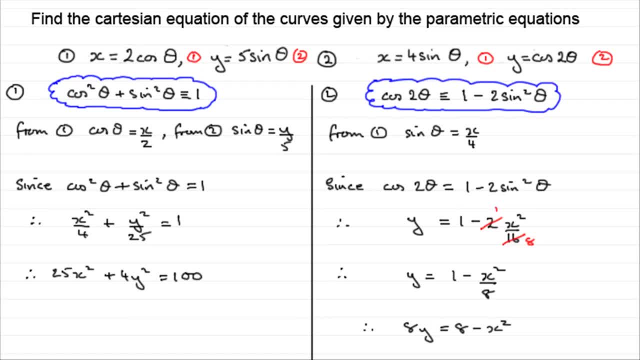 Look for an identity that links your trig functions together.